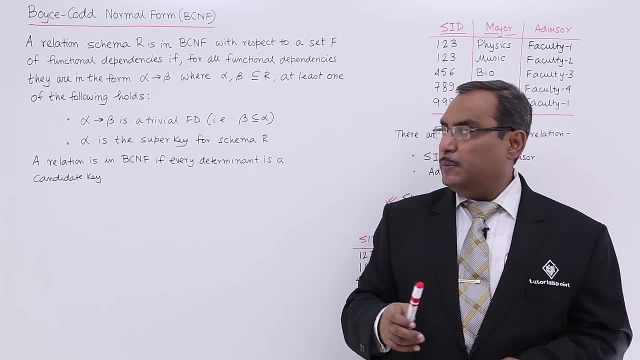 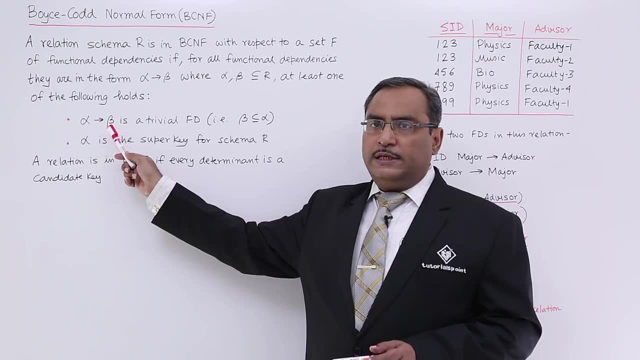 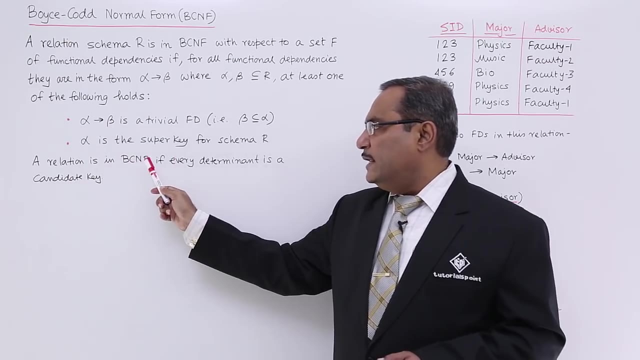 a tuple in a table is known as a super key for the respective table. So here alpha and beta are the set of attributes. Either this functional dependency will hold good. alpha is a super key for the schema capital R. A relation is in BCNF. if every determinant 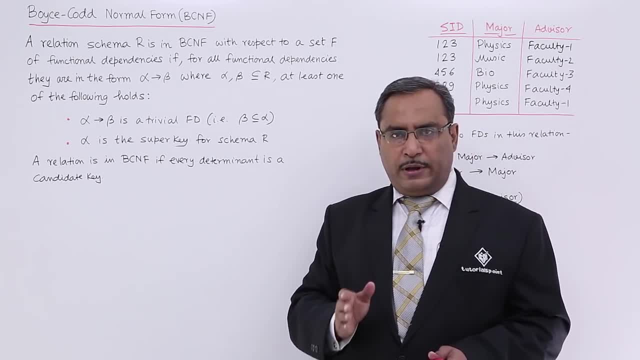 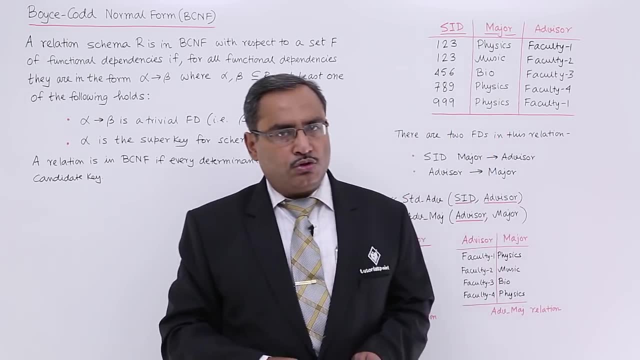 is a candidate key. So determinant means whatever coming on the left hand side of the functional dependency will be known as the determinant. So for the better understanding, let us go through one example. So this is one table where having the student id, where 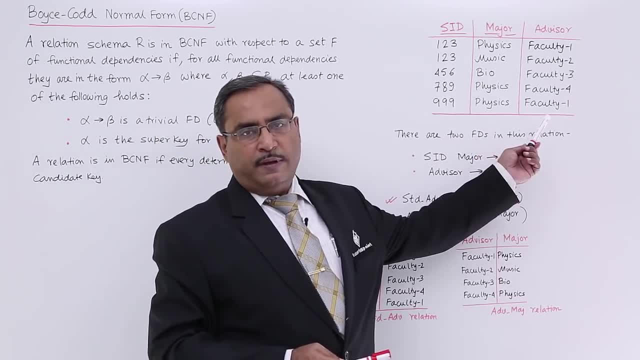 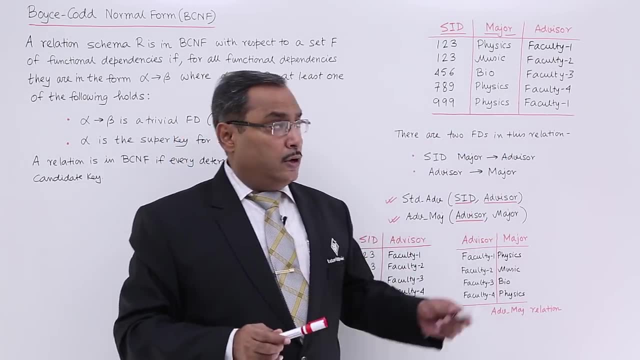 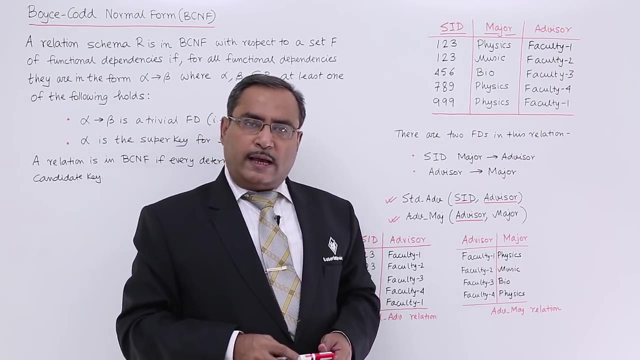 having the respective subject, that is major, and the respective advisor or the faculty details are there. So student id, major and advisor. This particular table is having multiple tuples are there, but there are some constraints, are there? Issue number one: a subject can have multiple advisors. Look at the physics. it is having faculty one also. 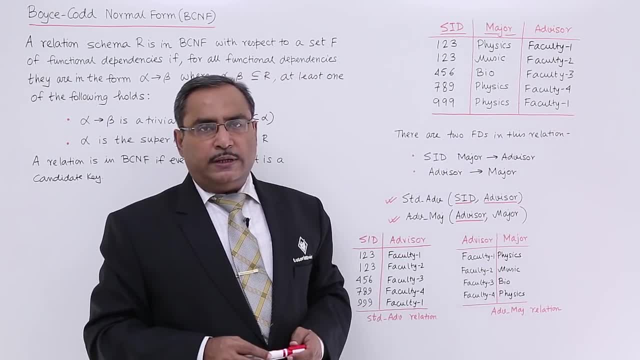 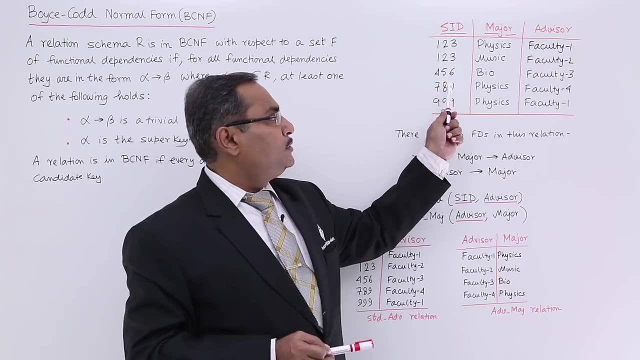 it is having faculty four. For a single subject there may be multiple students got registered. You can go for, say, physics. you see, for the single subject multiple students have got registered. So that is our issue number two. Issue number three: a faculty can teach. 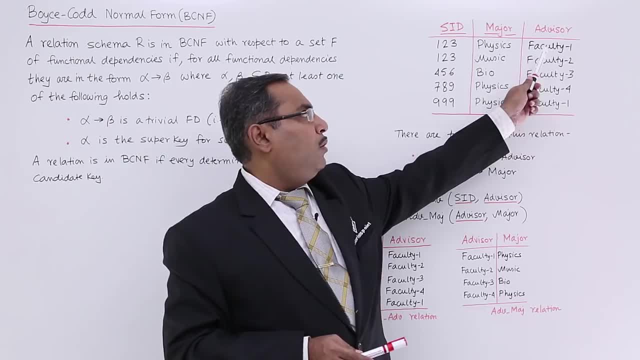 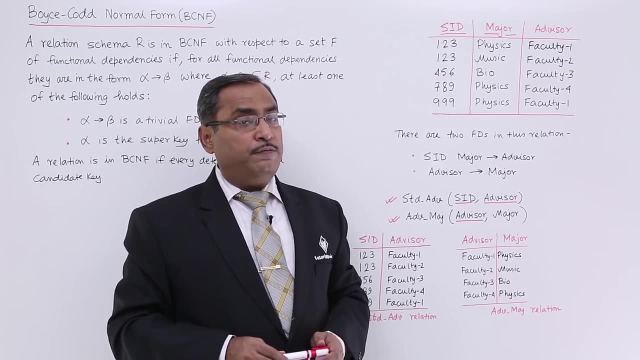 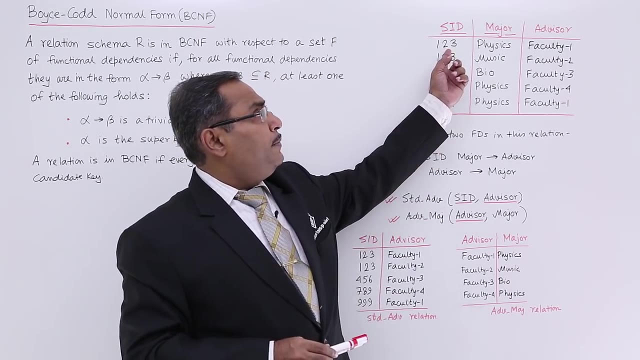 only one major. If you go for faculty number one, always he or she is teaching physics. So issue number four, for a single major, a student can take help from a single faculty. So whenever I am getting this one, two, three for the subject physics, I am getting a single. 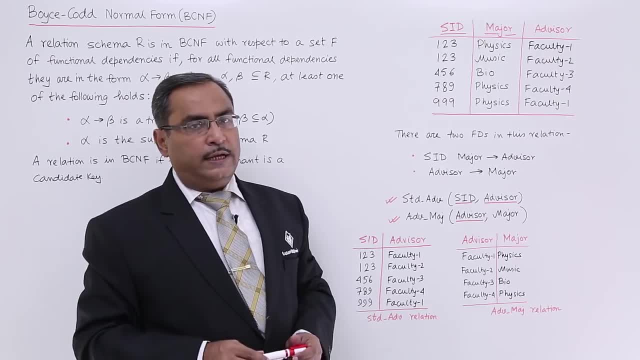 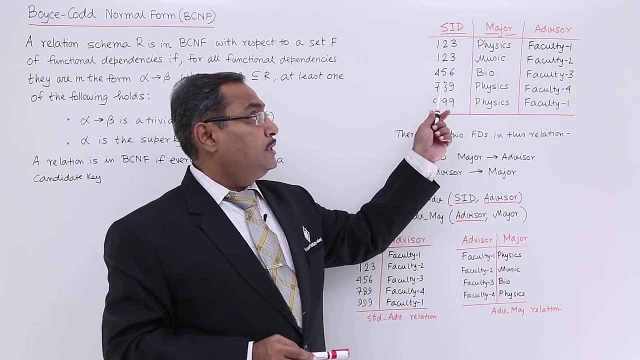 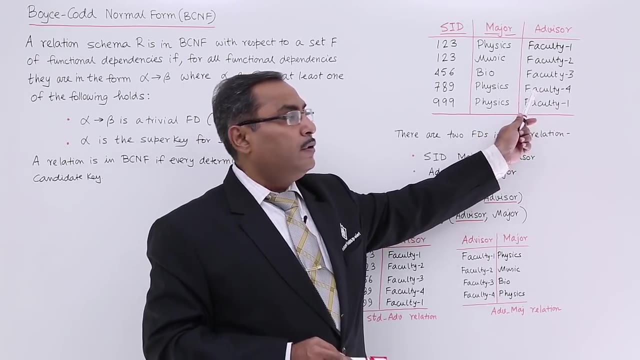 faculty name. that is, no other alternatives. And the issue number five is that for a single subject, as we are having multiple number of students, then for a single subject we can have multiple number of faculties also. So physics is being taught by faculty one, faculty four, both. So these are the five issues. 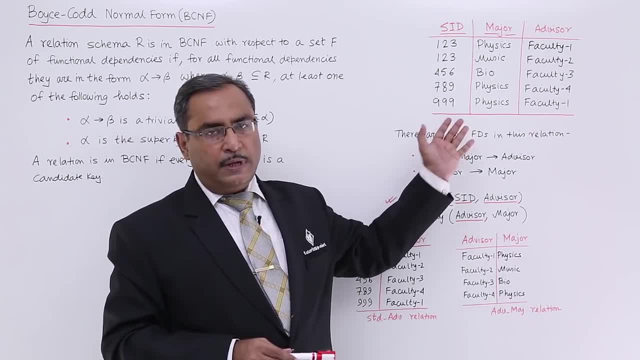 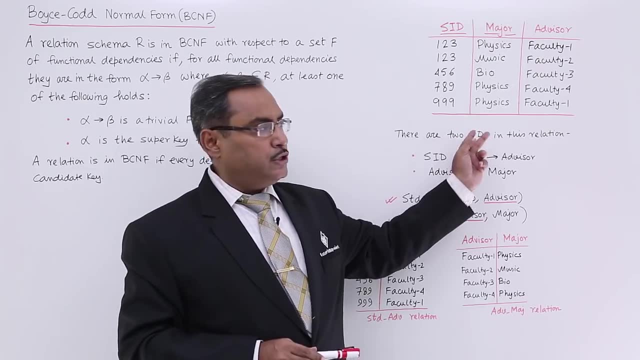 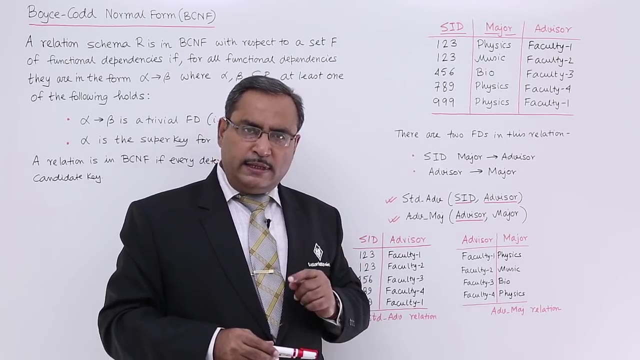 are there on which this particular table has been filled up, Keeping all those five issues. we are having two functional dependences from this particular relation. One is your student ID: major determines advisor, Because I told you that a student for a single subject. 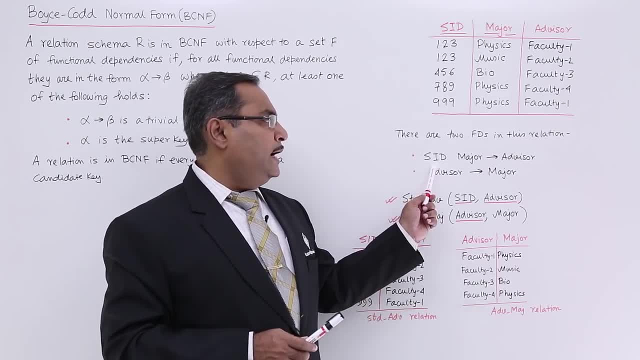 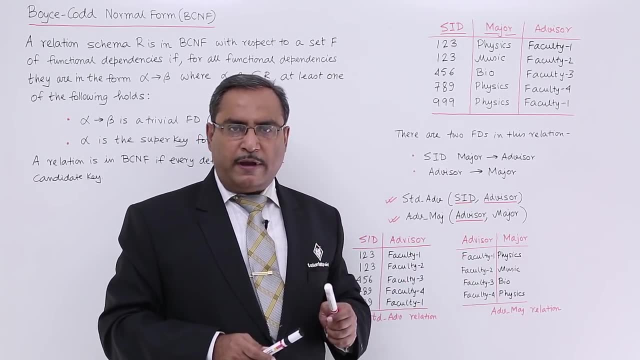 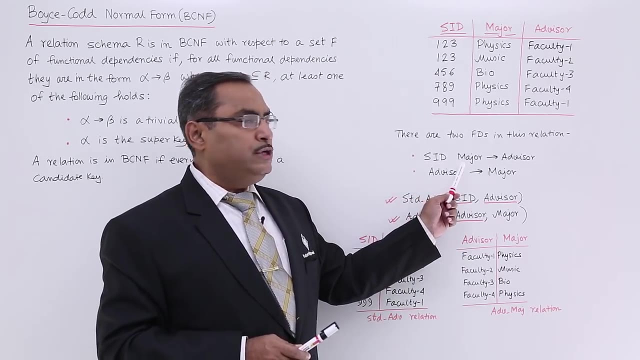 can take guidance from a single faculty. So student ID major determines advisor and advisor determines major. I told you this one, that a single faculty can give guidance to a single major only, a single subject only. So student ID major determines advisor and advisor determines major. So these two functional. 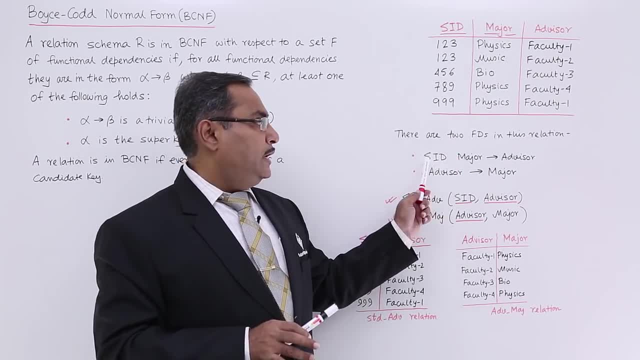 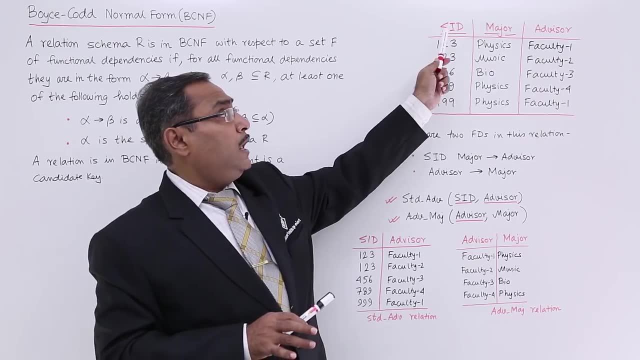 is we are having, we have derived from this relation. So here, student id and this major, they are the prime attributes, So they are forming a, they are forming a respective primary key. So that is, they are forming the respective composite key because more than one attributes. 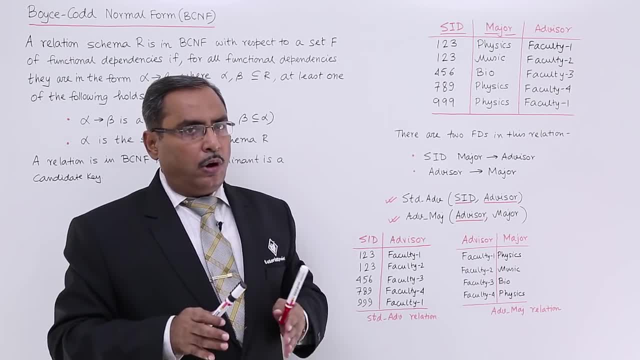 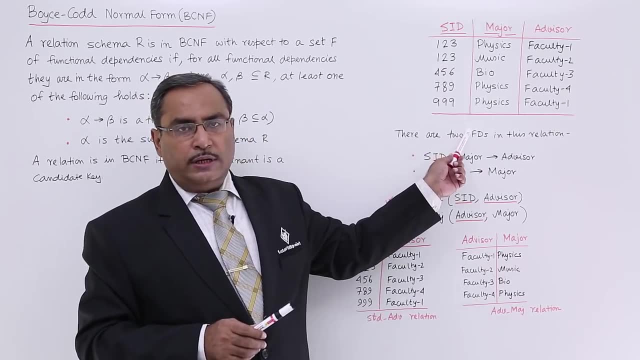 if they are forming a primary key, then the primary key can also be called as a composite key. So these are the prime attributes and this is a non prime attribute. So you see, this relation is in 1NF because there is no non-atomic data at the intersection of rows. 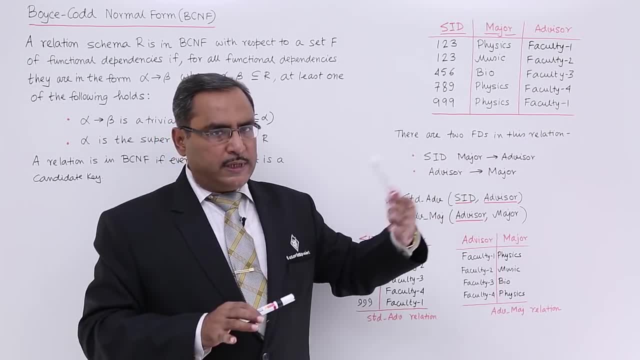 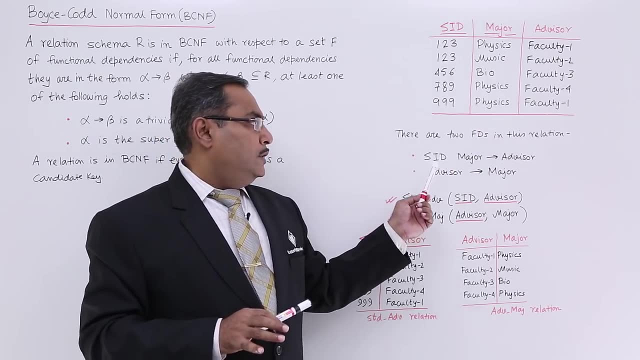 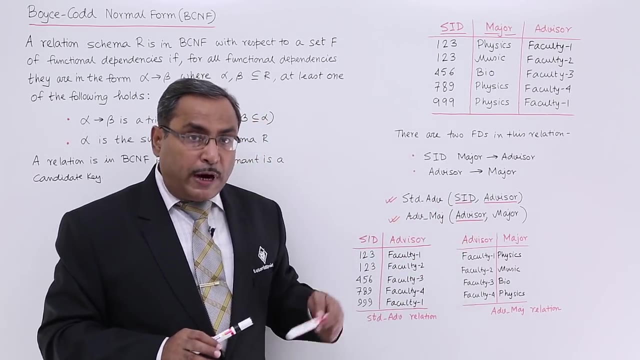 and columns and there is no repeating groups. So we have discussed it, this one in the in the respective video also. So this relation is in 1NF Now. student id major determines advisor. but I am not finding any other functional dependency, which is having the partial dependency. 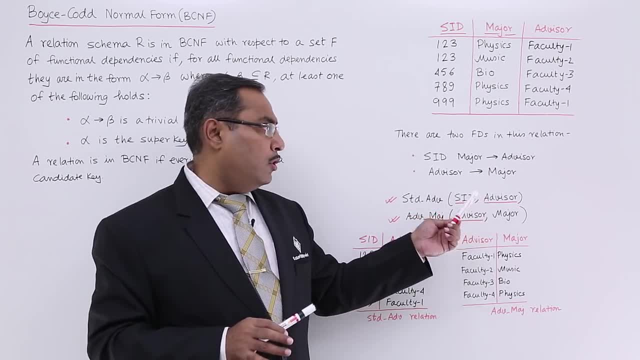 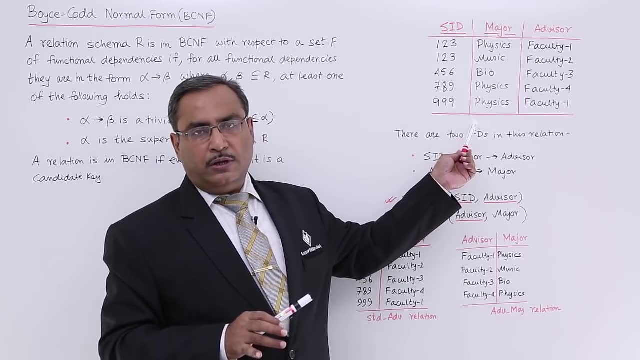 That means only major is determining some other attributes or only student id is determining some other attributes, or only student id is determining some other attributes or only student id is determining some other attributes. So there is no partial dependency. So this particular relation is also in 2NF Now student id, major determines advisor, but I am not. 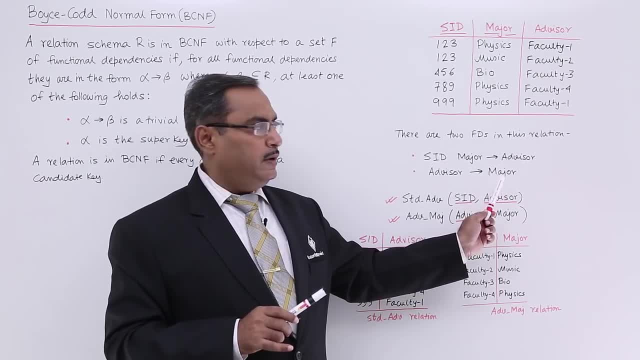 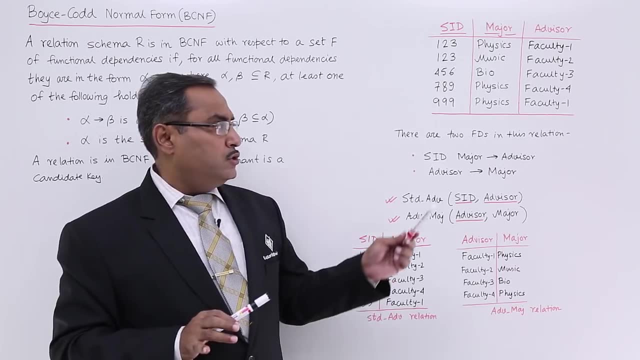 finding any other. I am not finding any other functional dependency. but advisor is determining another non-key attribute, So there is no transitivity here. So transitivity dependency is not here. So as there is no transitivity dependency, So that is why I am not finding. 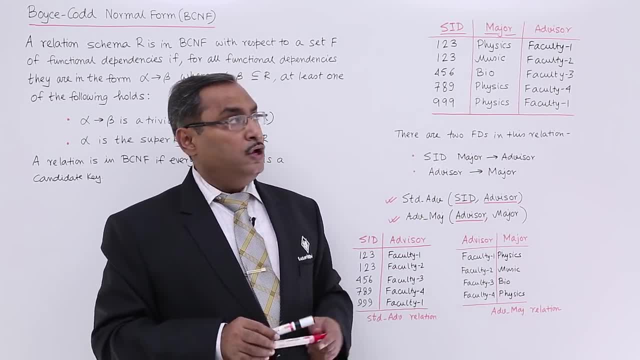 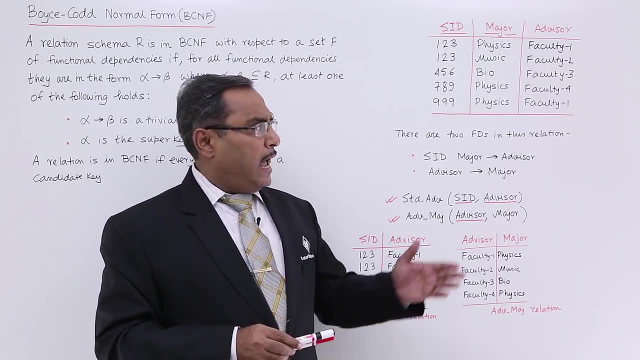 any other functionality here. We can see this here is useful for review Number one. it is using kinds of layouthhhwhy it is using a general layout that I saw in lecture number four that, if I enable, any other height linking system I am not finding. 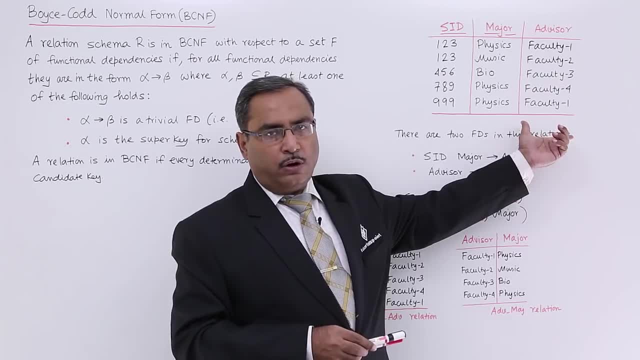 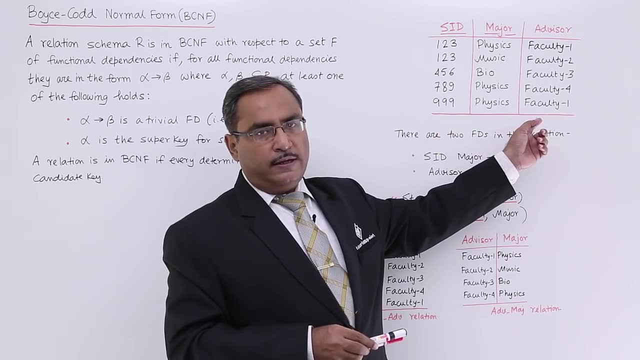 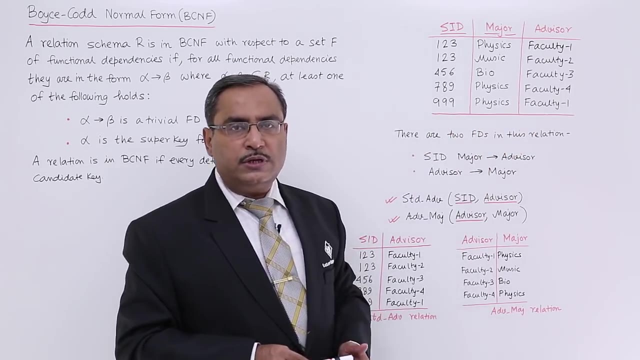 any other. des rugged alt logo behind tel is used here So termily in this part of the text and I will show you some details about survey anywhere. but for now the paper faculty details cannot be entered here because i cannot keep this key attributes prime attributes. 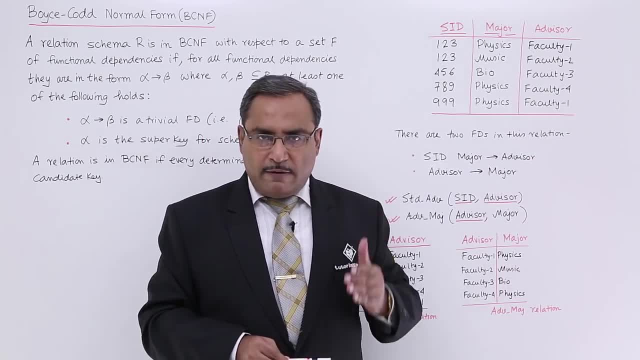 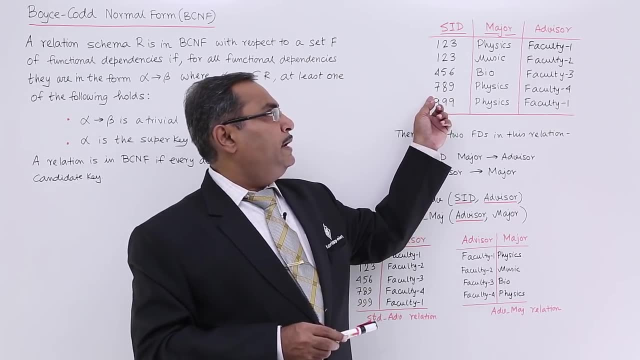 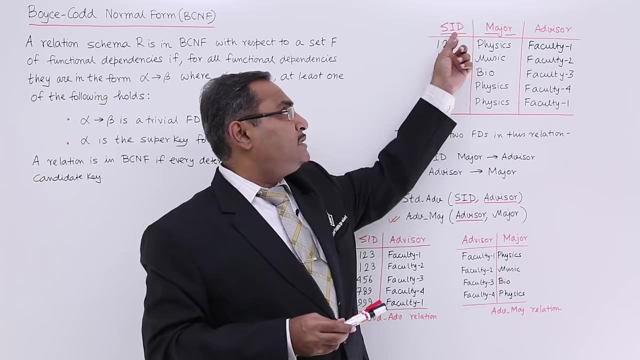 null, only just keeping the faculty name under the advisor attribute. so insertion anomaly is there. let us suppose this particular student 789 has taken tc, so he is going to another college due to some reason. so i cannot keep this student id null, so i should delete this record. so when? 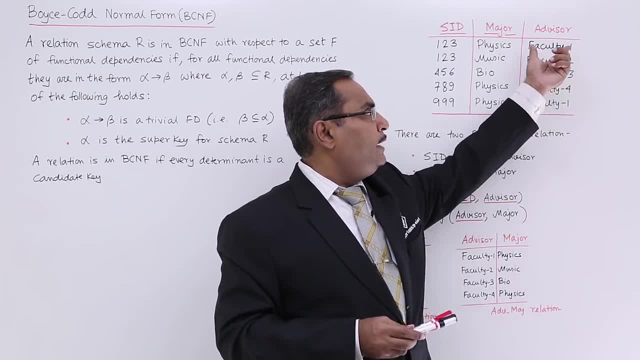 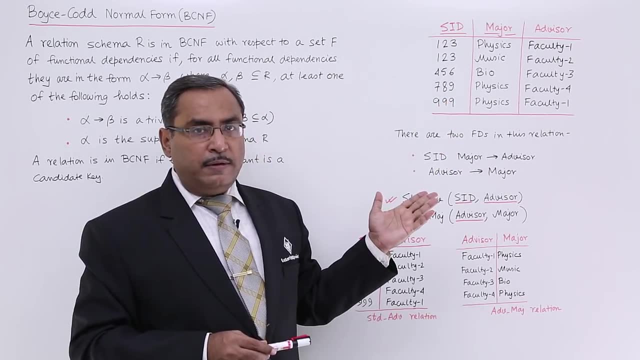 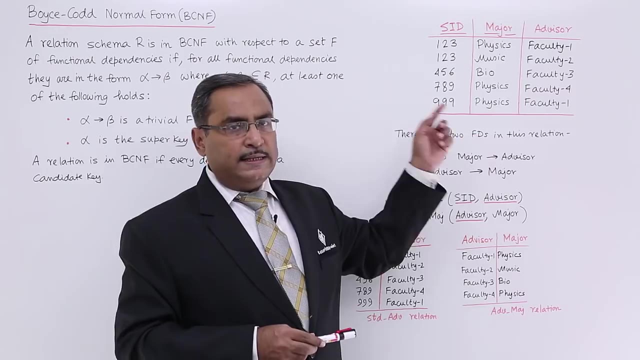 i am deleting this record. faculty number four will get deleted because faculty number four was having only one student and the student id was 789. so deletion anomaly is there. so here you see, this relation is in 1nf, also in 2nf, also in 3nf. still we are having anomalies on this particular relation. 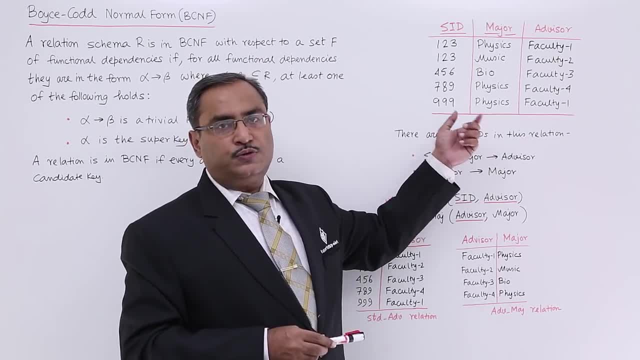 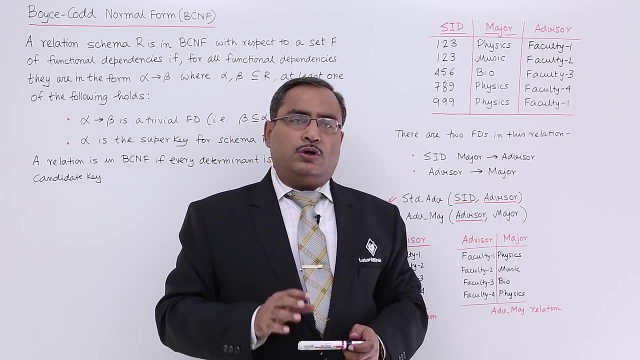 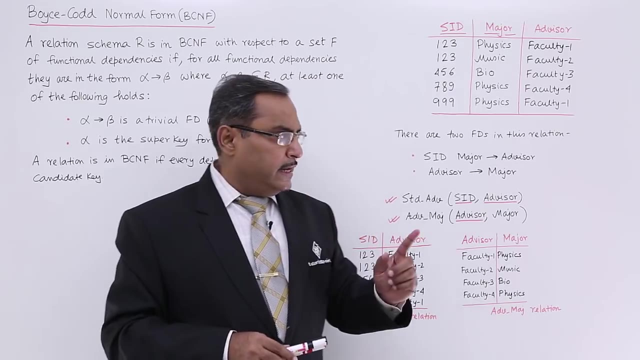 so i should, i should do something. i should split this table depending upon this functional dependencies, so that anomalies can be resolved. okay, how can i get that? this particular relation is not in bcnf? the thing is that whenever a non-prime attribute determines some of the prime attributes, 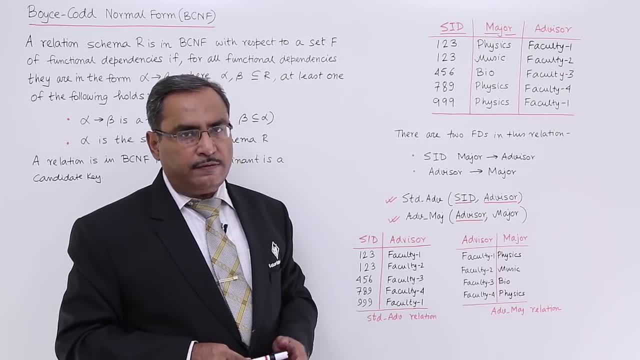 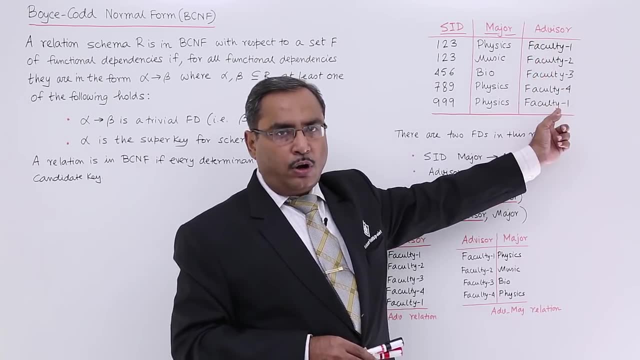 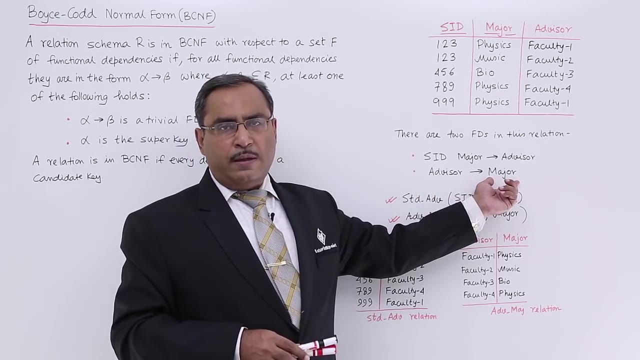 then we shall say that this relation is not in bcnf. again, i am repeating: whenever a non-prime attribute- because you see advisor is not underlined, so it is a non-prime attribute, whenever it is a non-prime prime attribute is determining one or more than prime attributes, then we shall say that. 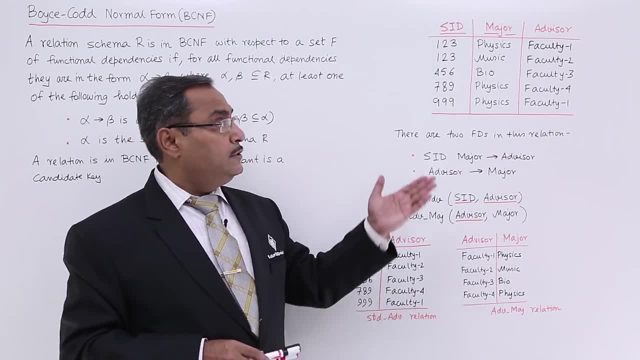 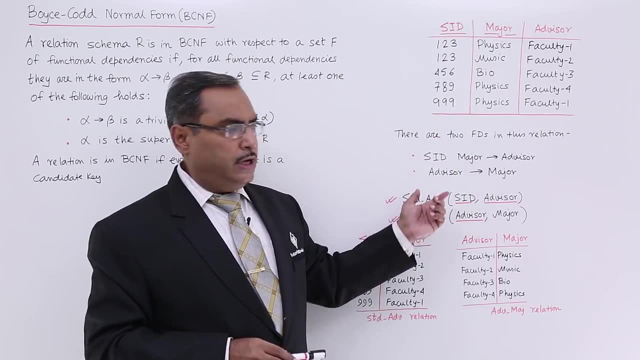 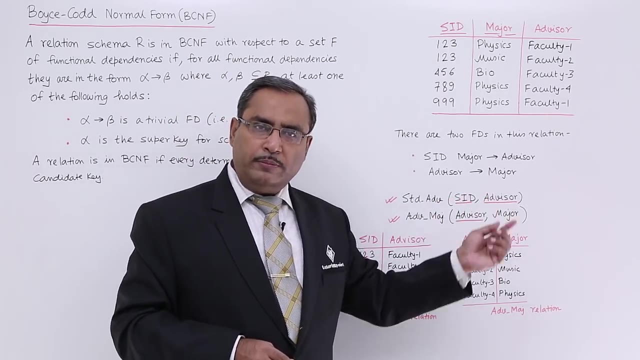 the relation is not in BCNF and we will be having so many anomalies in the respective relation. So now we are going to split this relation into two, into two relations. one is your student advisor, that is, the student id and the advisor, where both will become the prime attributes, and another one is the advisor major, where 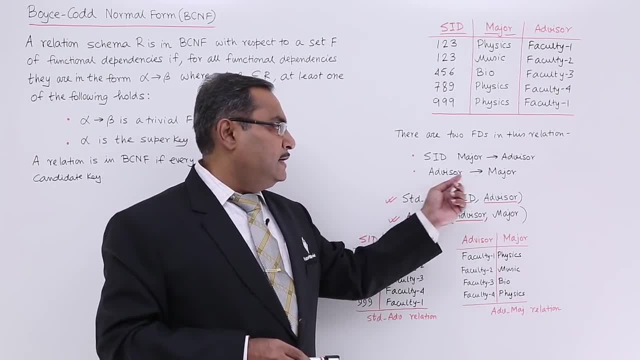 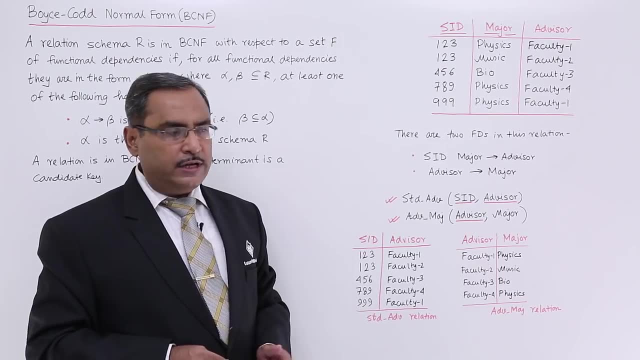 advisor will be the prime attribute and major will be coming, So advisor, major. So I am forming this one and from this particular functional dependency I shall form this student advisor relation. So two relations we are forming after splitting the, the mother one.